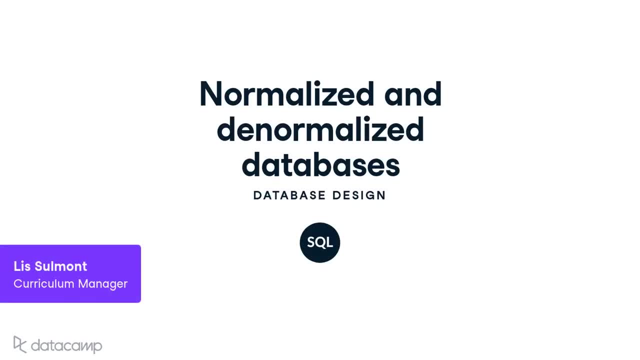 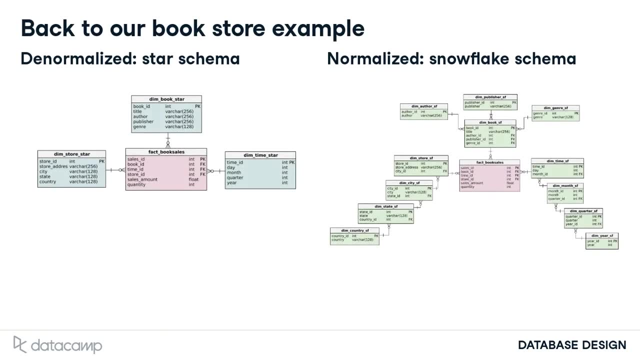 Welcome back. Now that we have a grasp on normalization, let's talk about why we would want to normalize a database. You should be familiar with these two schemas by now. They're both storing fictional company data on the sales of books in bulk to stores across the US and Canada. 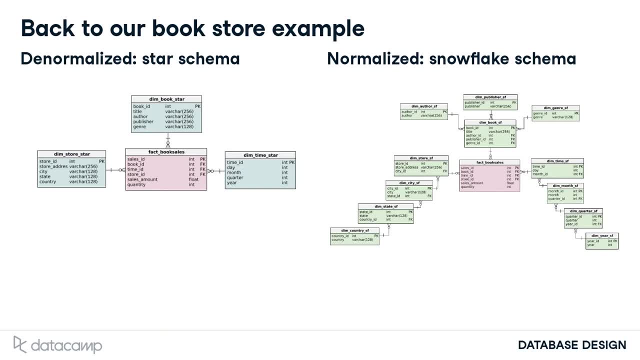 On the left you have the star schema with denormalized dimension tables and on the right you have the snowflake schema with normalized dimension tables. The normalized database looks way more complicated and it is in some ways. For example, let's say you wanted to get the quantity of all books by Octavia E Butler sold in Vancouver in Q4 of 2018.. 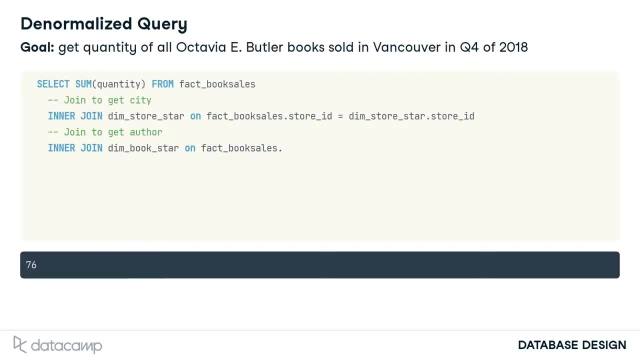 Based on the denormalized schema. you can run the following query to accomplish this. It's composed of three joins, which makes sense based on the three dimension tables in the star schema. What would the query look like on the normalized schema? A lot longer. 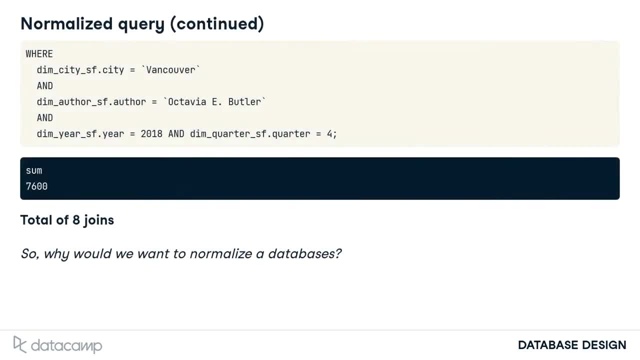 It doesn't even fit on the star schema. It only fits on one slide. There's a total of eight inner joins. This makes sense based on the snowflake schema diagram. The normalized snowflake schema has considerably more tables. This means more joins, which means slower queries. 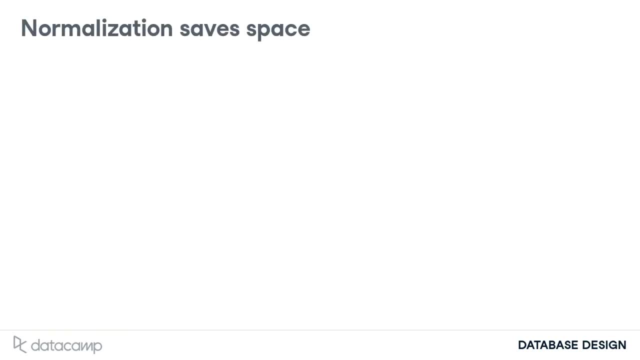 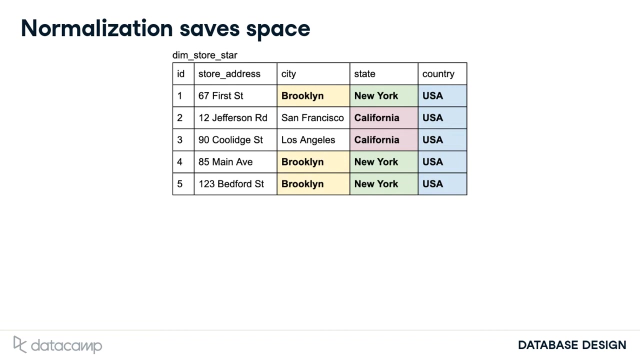 So why would we want to normalize a database? Normalization saves space. This is an intuitive seeing how normalized databases have more tables. Let's take a look at the store table in our denormalized database. Here we see a lot of repeated information in bold, such as USA, California, New York and Brooklyn. 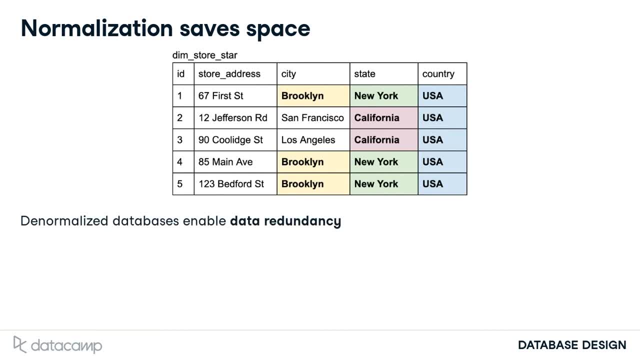 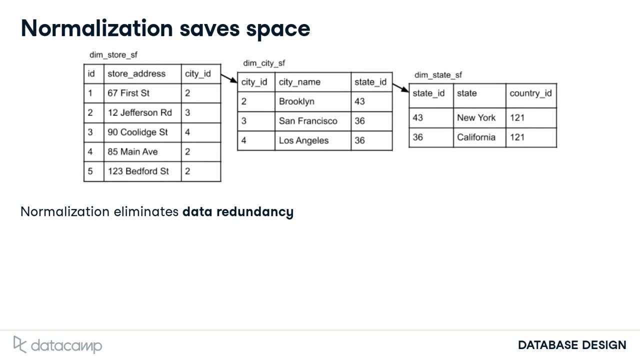 This type of denormalized structure enables a lot of data redundancy. If we normalize that previous schema, we get this. We see that although we are using more tables, there is no data redundancy. The string Brooklyn is only stored once and the state records are stored separately because many cities share the same state and country. 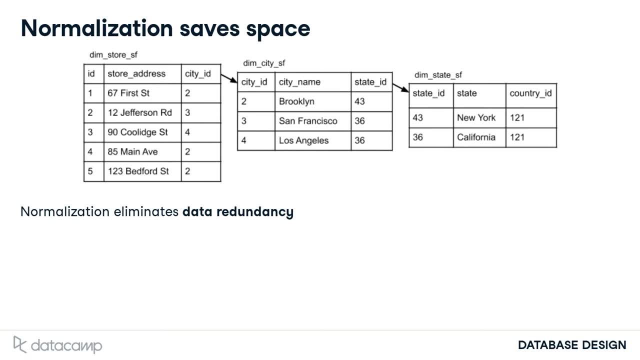 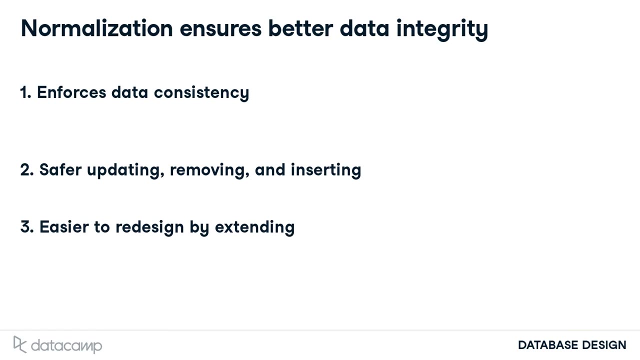 We don't need to repeat that information. Instead, we can have one record holding the string California. Here we see how normalization eliminates data redundancy. Normalization ensures better data integrity through its design. First, it enforces data consistency. Data entry can get messy and at times people will fill out fields differently.